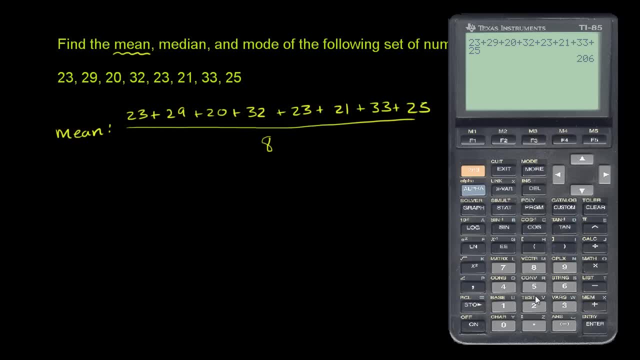 And then we want to divide 206 by 8.. So if I say 206.. 206 divided by 8 gets us 25.75.. So the mean is equal to 25.75.. So this is one way to kind of measure the center. 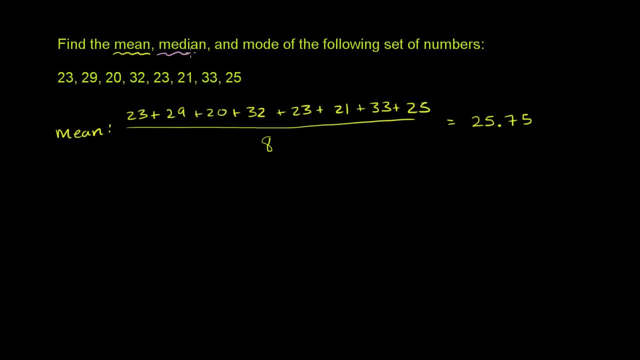 the central tendency. Another way is with the median, And this is to pick out the middle number, the median, And to figure out the median. what we want to do is order these numbers from least to greatest, So it looks like the smallest number here is 20.. 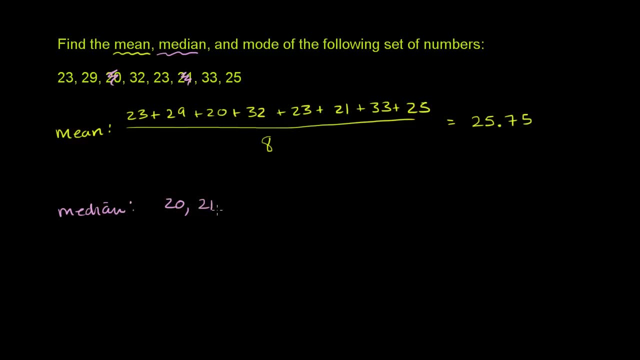 Then the next one is 21.. Then we go: there's no 22 here. There's, let's see, there's two 23s, 23 and a 23. So 23 and a 23. And no 24s. 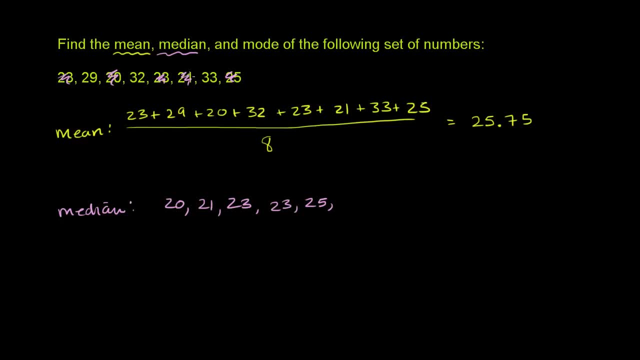 There is a 25.. There's no, 26,, 27,, 28.. There is a 29.. Then you have your 32. And then you have your 33.. So what's the middle number, now that we've ordered it? 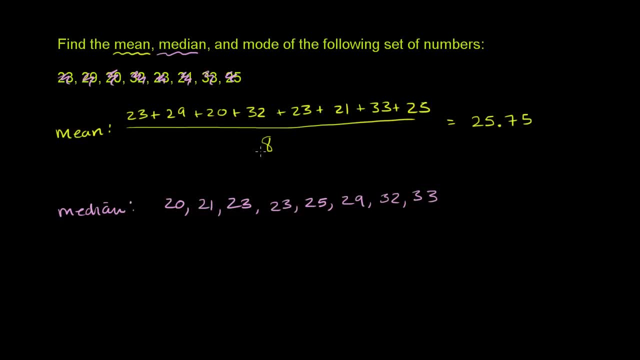 So we have 1,, 2,, 3.. 4.. 4,, 5,, 6,, 7,, 8 numbers. We already knew that, And so there's actually going to be two middles. If you have an even number, there's. 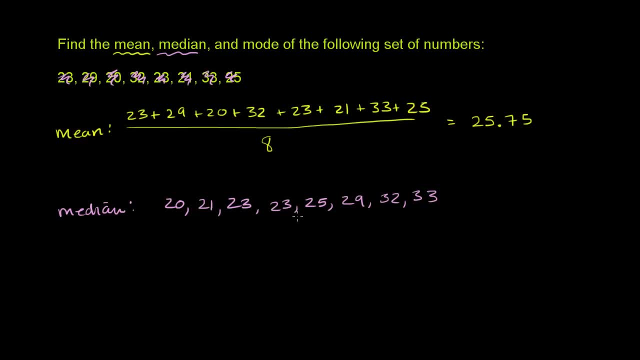 actually two numbers that kind of qualify for the close to the middle And to actually get the median, we're going to average them, So 23 will be one of them. That by itself can't be the median, because there's 3 less than it and there's 4 greater than it. 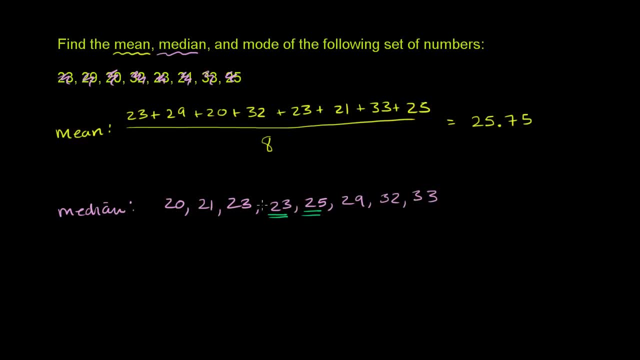 And 25 by itself can't be the median because there's 3 larger than it and 4 less than it. So what we do is we take the mean of these two numbers and we pick that as the median. So if you take 23 plus 25 divided by 2,, 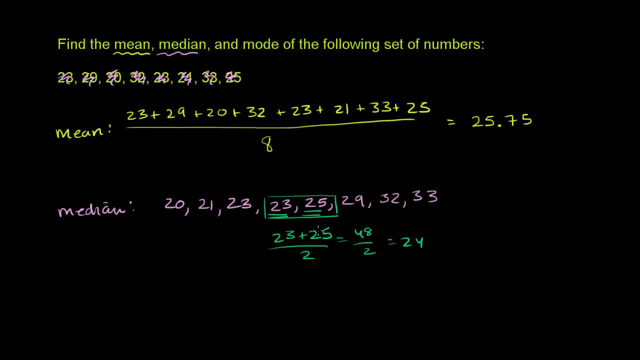 that's 48 over 2,, which is equal to 24.. So, even though 24 isn't one of these numbers, the median is 24.. So this is the middle number. So once again, this is one way of thinking about central tendency. 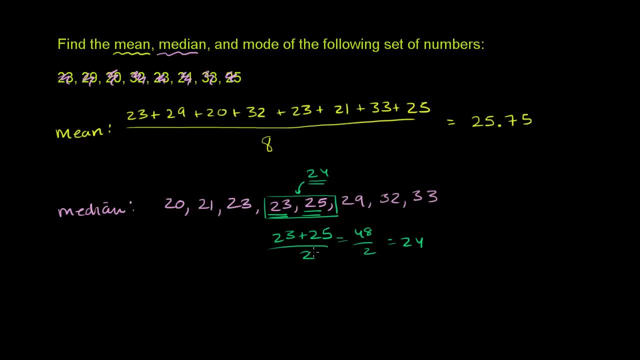 If you wanted a number that could somehow represent the middle, And I want to be clear, there's no one way of doing it. This is one way of measuring the middle. Let me put that in quotes: The middle. if you had to represent this data with 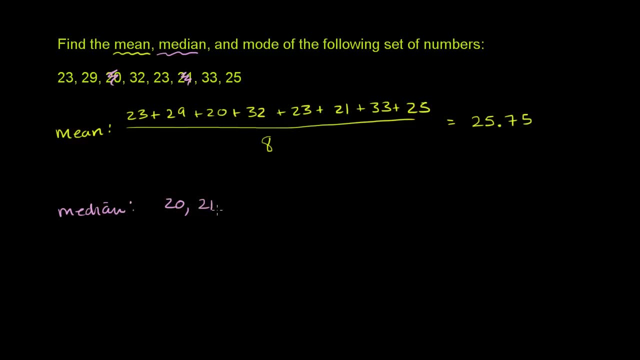 Then the next one is 21.. Then we go: there's no 22 here. There's, let's see, there's two 23s, 23 and a 23. So 23 and a 23. And no 24s. 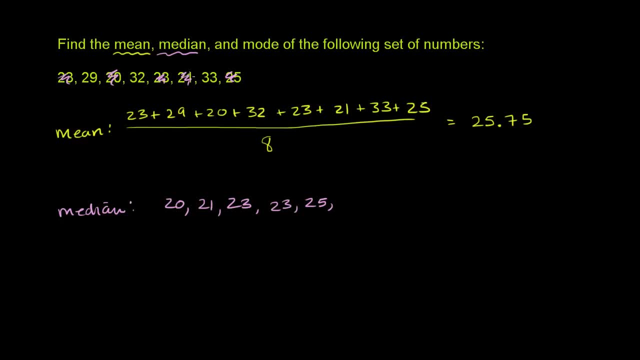 There is a 25.. There's no, 26,, 27,, 28.. There is a 29.. Then you have your 32. And then you have your 33.. So what's the middle number, now that we've ordered it? 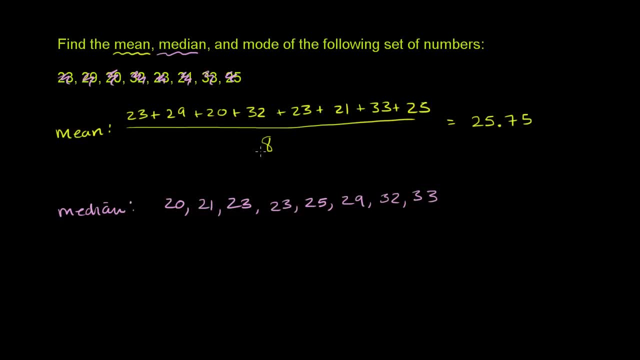 So we have 1,, 2,, 3.. 4.. 4,, 5,, 6,, 7,, 8 numbers. We already knew that, And so there's actually going to be two middles. If you have an even number, there's. 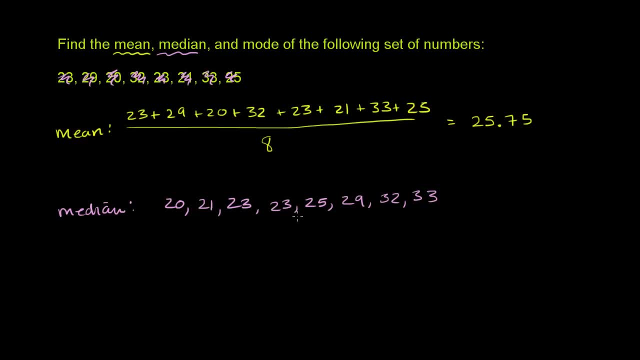 actually two numbers that kind of qualify for the close to the middle And to actually get the median, we're going to average them, So 23 will be one of them. That by itself can't be the median, because there's 3 less than it and there's 4 greater than it. 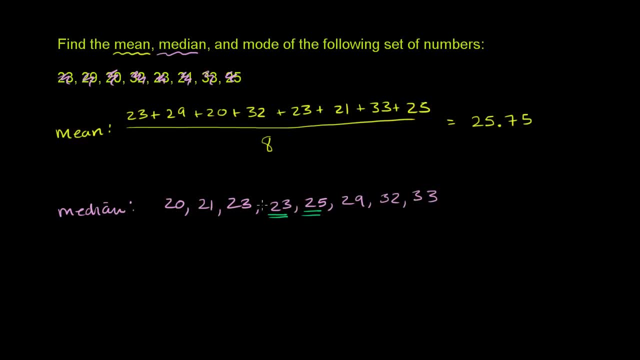 And 25 by itself can't be the median because there's 3 larger than it and 4 less than it. So what we do is we take the mean of these two numbers and we pick that as the median. So if you take 23 plus 25 divided by 2,, 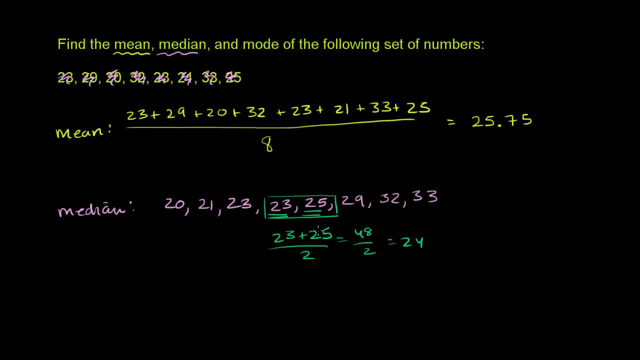 that's 48 over 2,, which is equal to 24.. So, even though 24 isn't one of these numbers, the median is 24.. So this is the middle number. So once again, this is one way of thinking about central tendency. 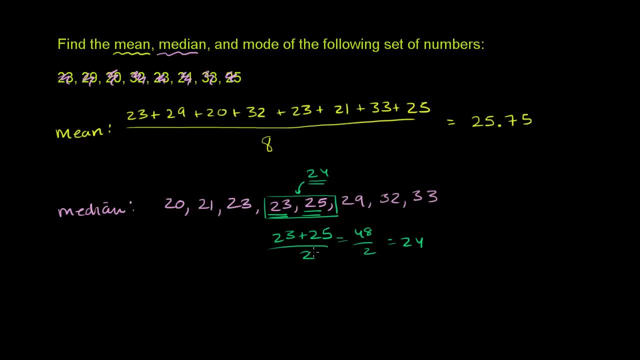 If you wanted a number that could somehow represent the middle, And I want to be clear, there's no one way of doing it. This is one way of measuring the middle. Let me put that in quotes: The middle. if you had to represent this data with 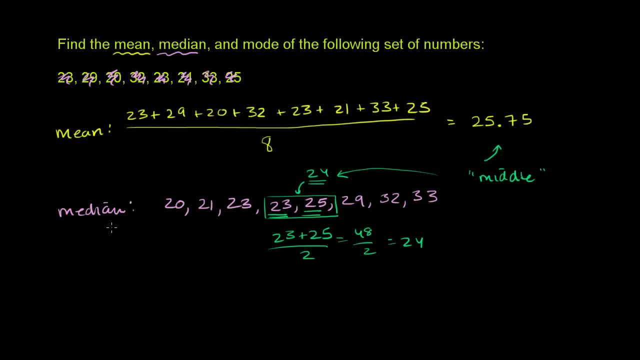 one number, and this is another way of representing the middle. Then, finally, we can think about the mode, And the mode is just the number that shows up the most in this data set, And all of these numbers show up once, except we have the 23.. 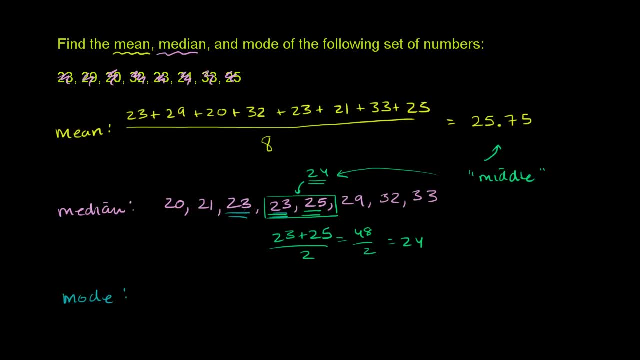 It shows up twice, And so because 23 shows up the most, it shows up twice. Every other number only shows up once. 23 is our mode.